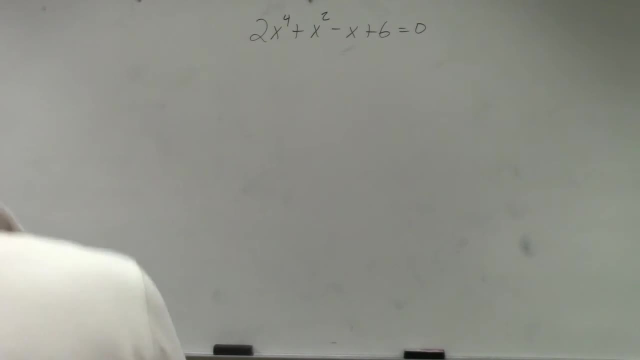 Asking us to determine the number of possible real, rational, real, negative, I'm sorry. positive, real, negative, real and then complex zeros, correct Descartes, rule of sines. So that's all I wanted you guys to do. So, if you guys remember for this, to find the positive all. 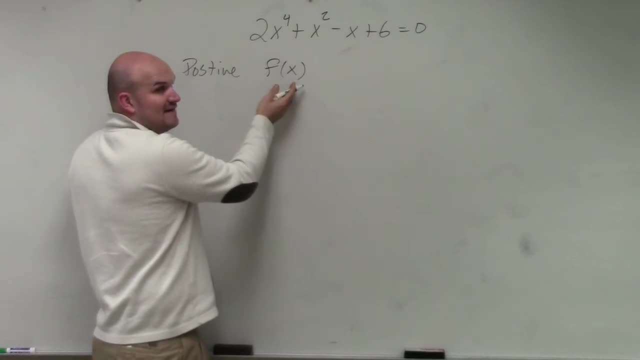 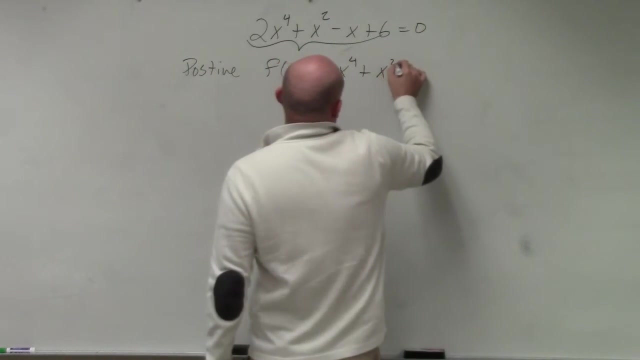 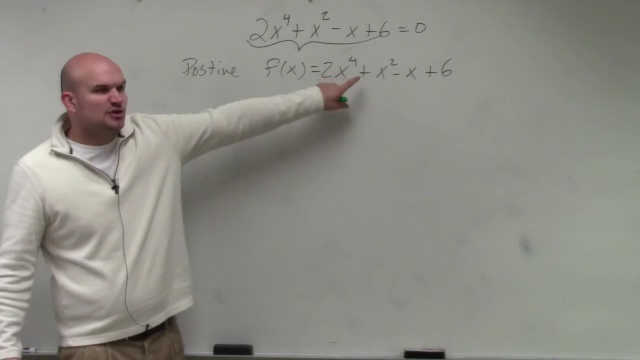 you're simply going to do is take f of x, find the number of sine changes of f of x. So f of x basically just represents the polynomial 2x to the fourth plus x, squared minus x plus six For long division and synthetic division. if we were missing a term, we included zero. 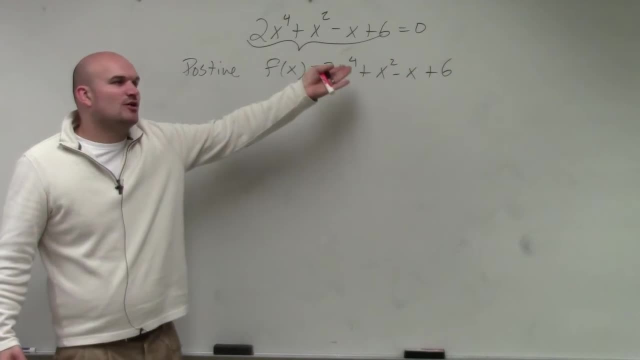 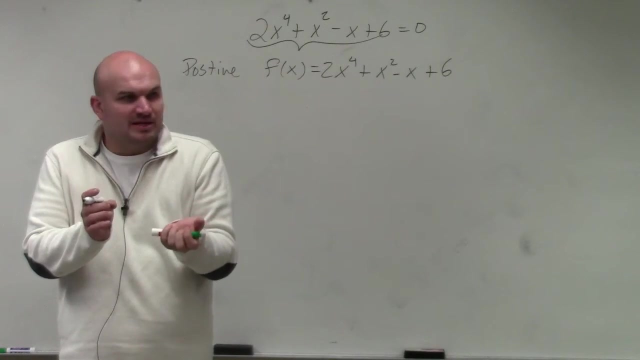 x. right, But we just wrote it as plus zero x. But, ladies and gentlemen, plus zero or minus zero is the same thing. So we don't want to include a zero there, because it's not. actually, we don't know if zero is not positive nor negative, right, So you? 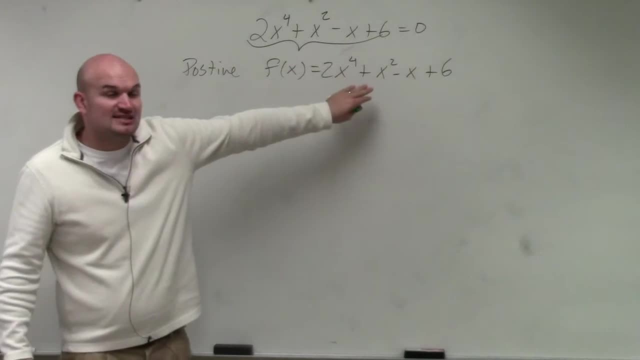 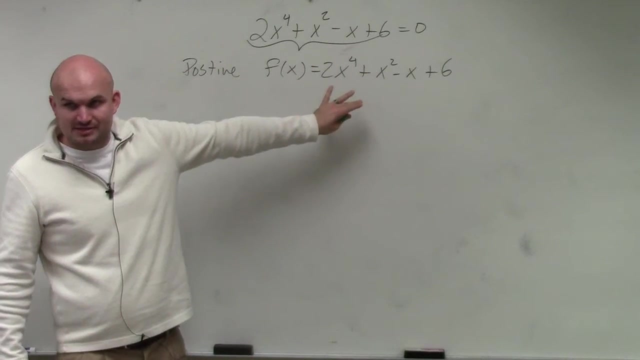 can't, so we don't need to include a zero. We need a zero for x cubed, So do not put zero x cubed. When we did division, you needed to do that. We don't need to do that for this. okay, So to find the number of positives, all you're doing is finding the number of. 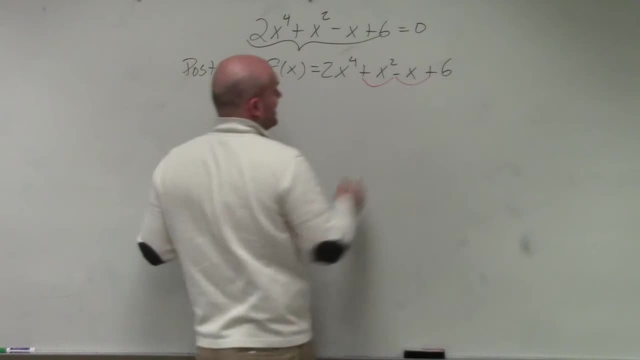 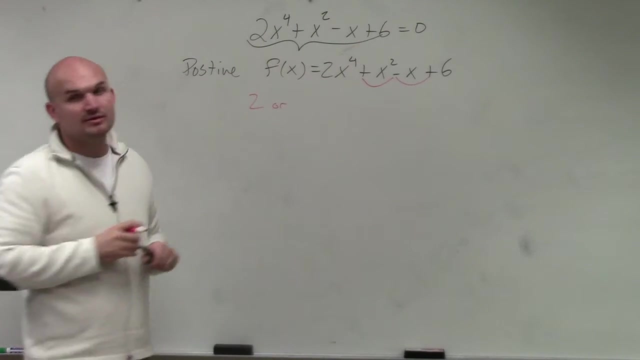 sine changes Anytime you go from positive to negative and negative to positive. Then you take the number of sine changes minus an even number. Well, even number, the basic definition of an even number- would be a number that's divisible by two, right, So you? 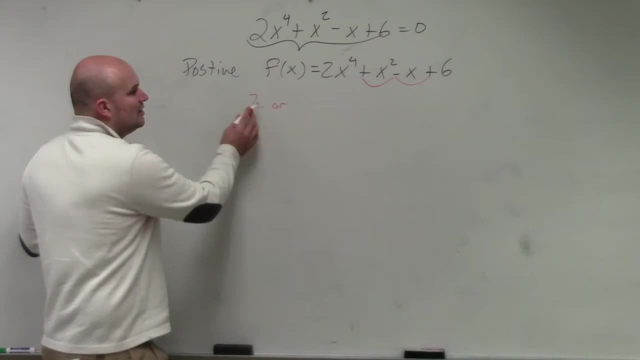 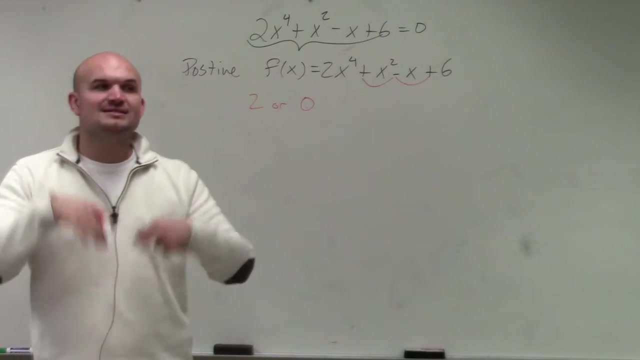 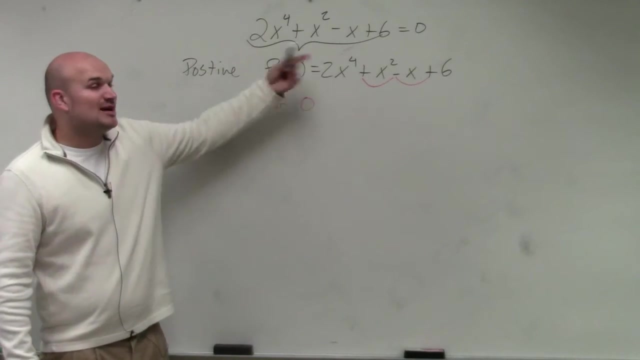 can't do that, So I always just like to divide by two as many times as I can. Well, if I divide, if I, sorry, not divide subtract by two as many times as I can, Excuse me, Two minus zero is. two minus zero is, I'm sorry. two minus two is zero If I subtract. 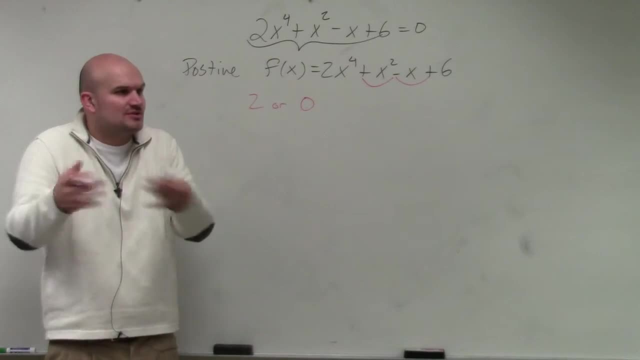 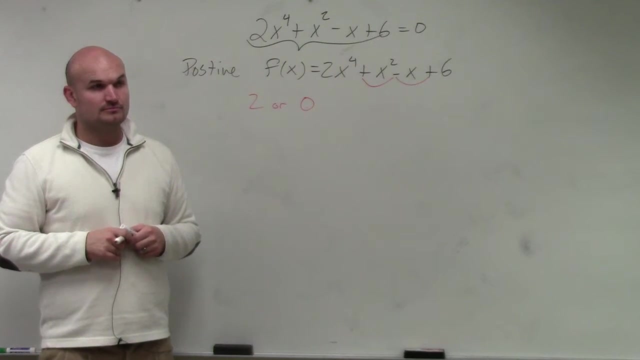 two. again, I'm going to get negative numbers. Well, I'm counting how many zeros are, So we can't have negative amount of zeros. So once we get to zero, that's it. Yes, So say you had four instead of two. 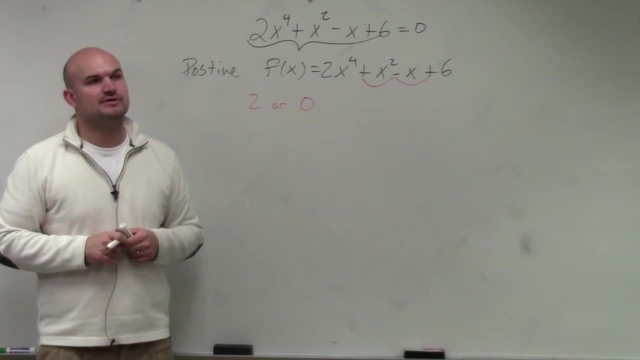 Four two zero Two minus two, Twice Yep. So it would be four two zero Four, two zero, Yep. Perfect, All right. So now usually everybody gets this one. This one's not too bad, Everybody has trouble with. 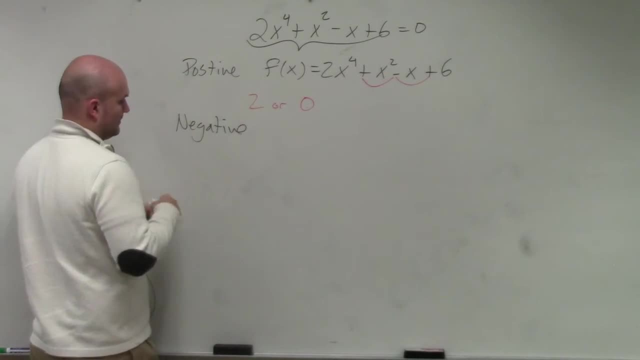 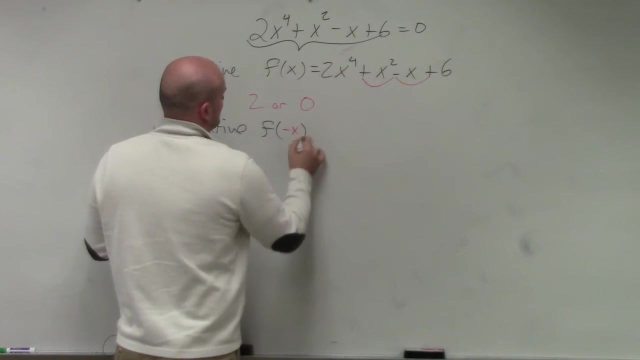 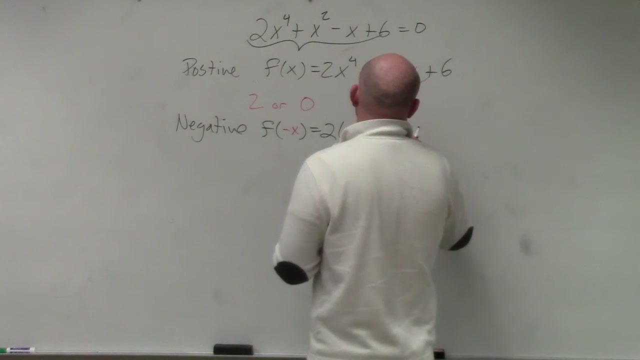 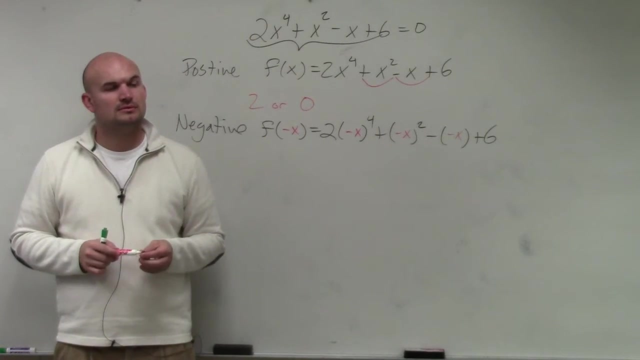 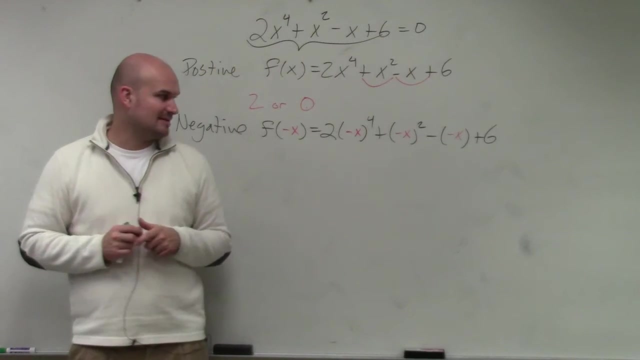 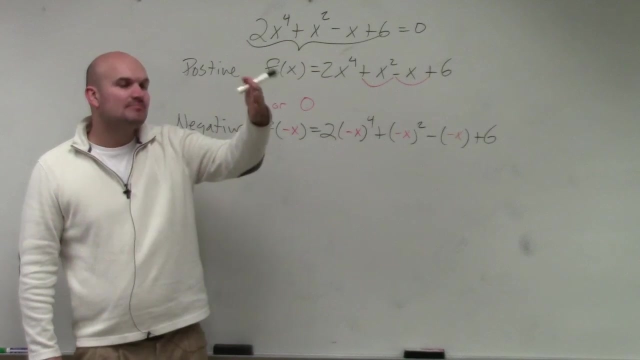 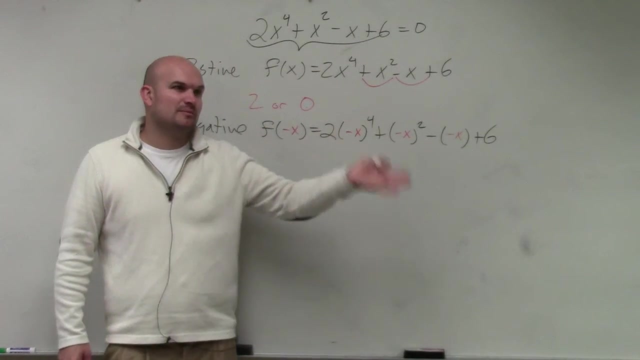 the negative. So that is f of now, negative x. Does everybody see that? Now, please remember, yes, So what I was just about to say is: any negative value raised to an even power is positive. Okay, Okay, Anytime. I wouldn't really say flip sign, because then you think you'd go from like always. 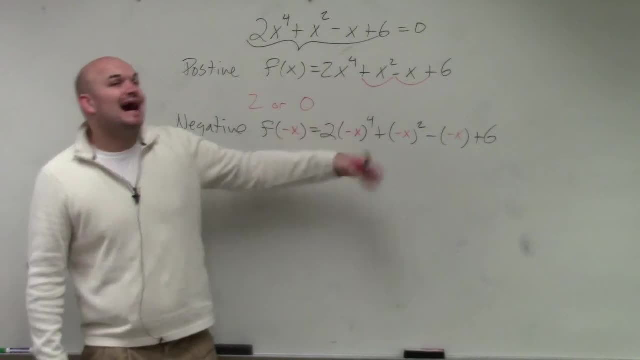 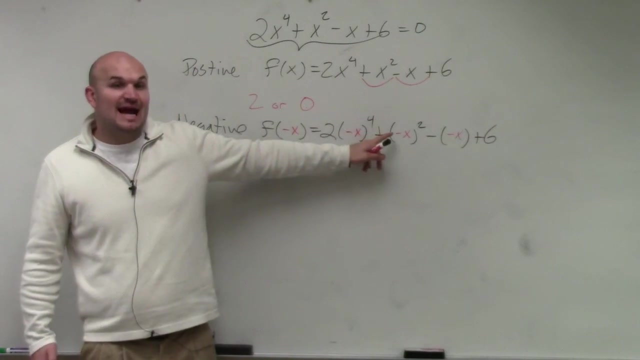 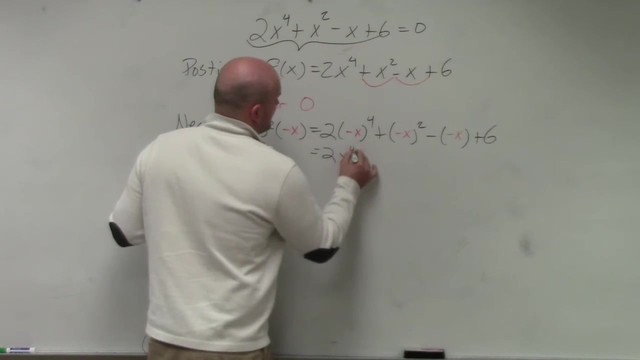 do the opposite. Any negative number raised to an odd power is always negative. Okay, So negative X to the fourth is going to be X to the fourth. positive X to the fourth. Positive X to the fourth times two is just positive two. X to the fourth, Negative X squared is now going to become a. 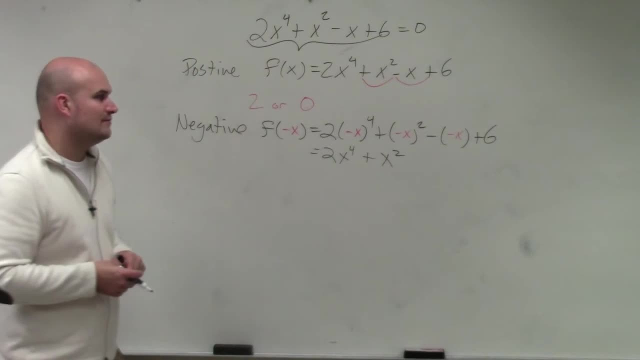 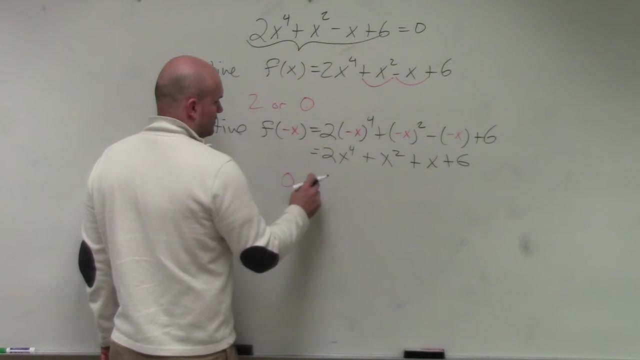 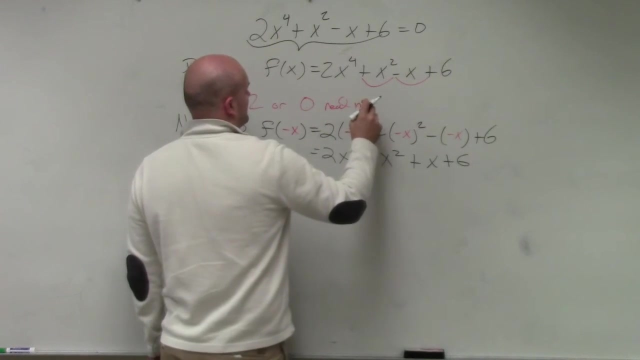 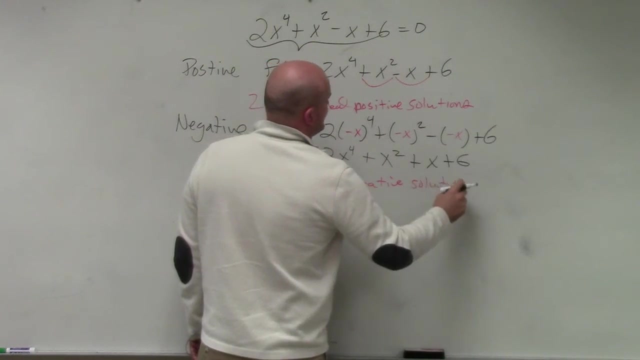 positive X squared Negative X times our negative, negative X is now a positive X plus six Right, So how many zero, how many real zero solutions do we have? Zero, right, All right. So what I wanted you guys to do, though, is to find out about the complex, So 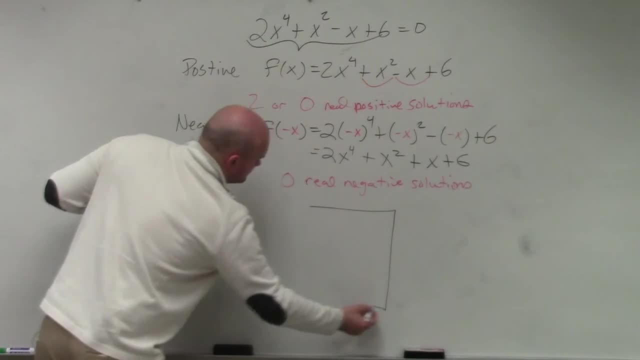 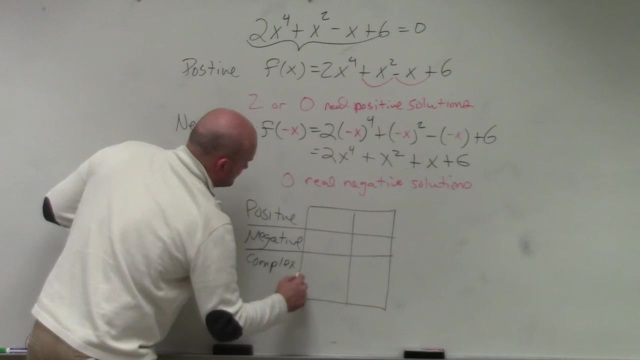 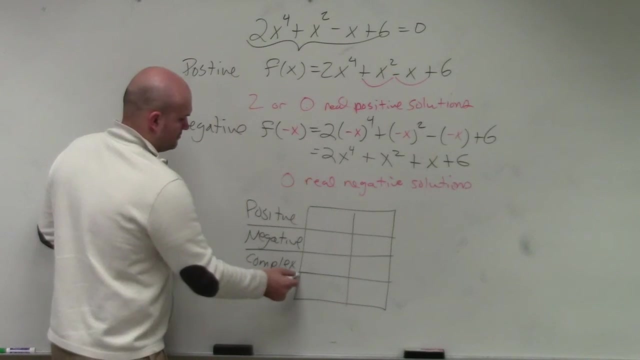 since I have two options here, I'm going to create two columns, So we want to figure out how many positive we have, how many negative, how many complex, And use the total amount. So how many positive do we say There's two options, right? 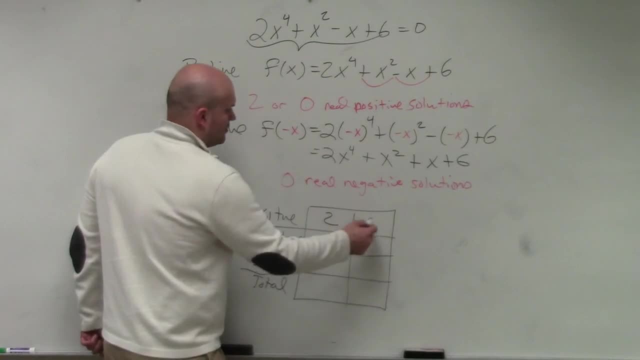 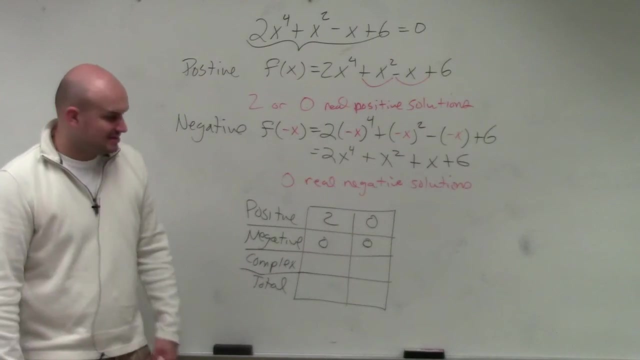 That's why I did two columns. So we have 2 or 0.. How many negative do we have 0. And before we get to complex, how many total is there? What's the degree? 4, right. So therefore we have 4 and 4..